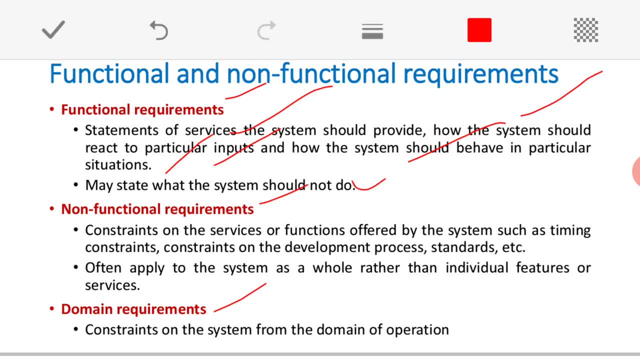 in defining what What my system should not do also ok. sometimes we need to tell that also explicitly in our requirement: that my system should not do like this. it is clear, ok, And what about the non-functional requirements? here The definition says that non-functional requirements are nothing but. 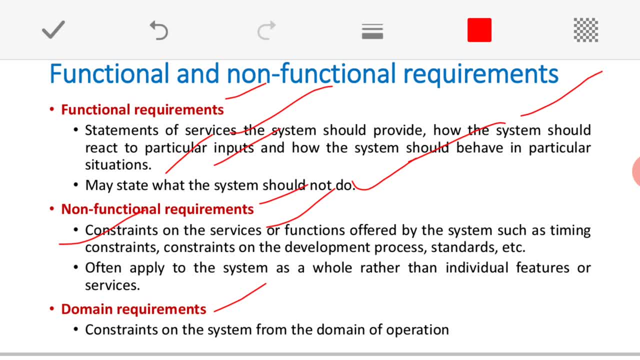 these are the constraints on the services or functions offered by the system, such as timing constraints- ok. the constraints on development process- the standards means the standards to be get adopted, or the budget or the cost of the software. cost of the money constraints- ok. And another important thing is whenever we will talk about the non-functional. 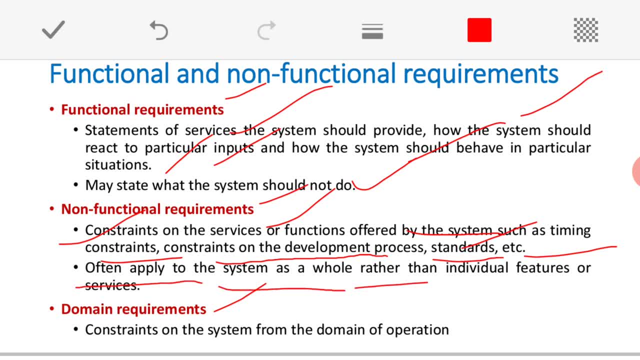 requirements are concerned, they are often applied to the system as a whole rather than what the individual features or services. ok, that is very important. So, especially this, non-functional requirements, for example, say, when I am talking about the timing constraints With respect to the performance, for example, so how I can define whether the performance 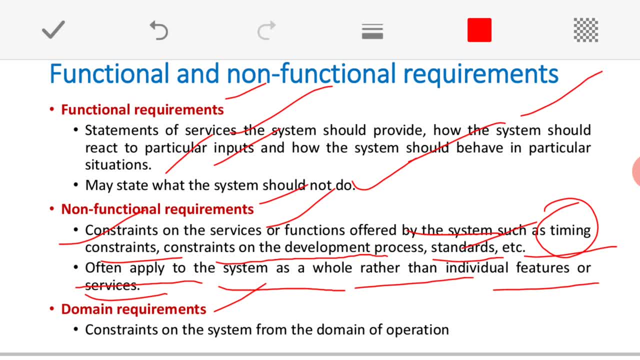 of my software is good or better or best or it is bad. ok, So whenever I am talking about the performance, normally I used to take the software as a whole, the full software. I used to talk about: ok, See, for example, if you take an example of the mobile. ok, so I will never talk about. 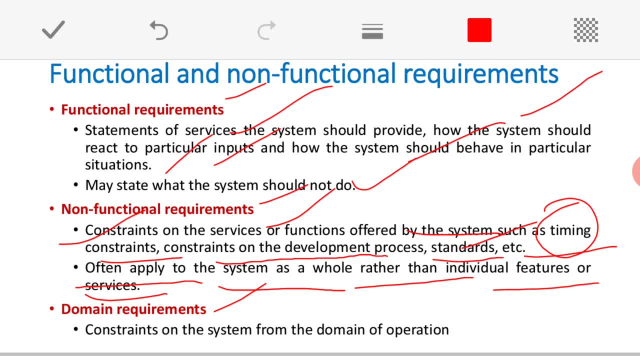 so finally, I need to conclude that. so what is the overall performance of my particular mobile? ok, I cannot simply talk about the performance, Ok, the individual component level. So the process is good or bad. ok, So whether the memory capacity is good or bad. So I cannot go with the individual part by part here. ok, So that. 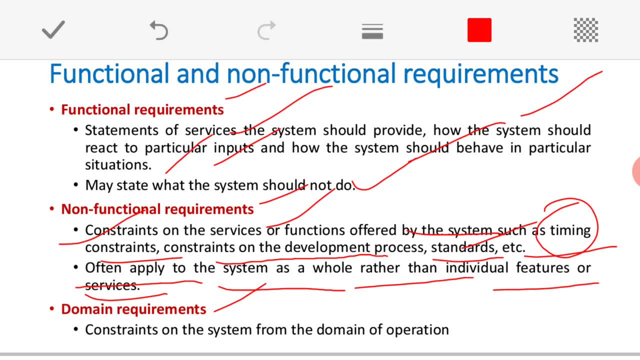 is nothing but what. that is the meaning of this, the system as a whole here. ok, Then the last type of the classification is that is domain requirement. So domain requirement means actually these are the requirement of the type of constraints on the system from: 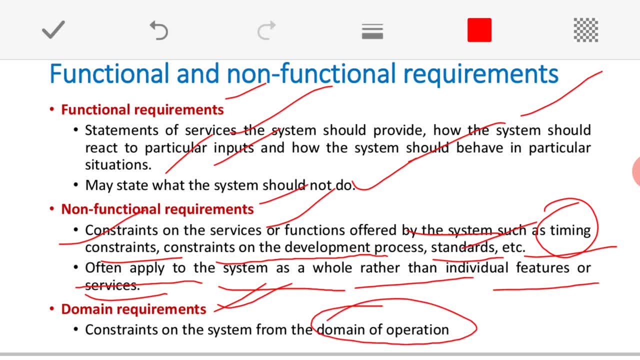 the domain of the operation. So here the domain in the sense. what always do remember today, whatever the software that we might be using, we are all using that software for a particular type of application. ok, For example, say today, if I am using one college automation- 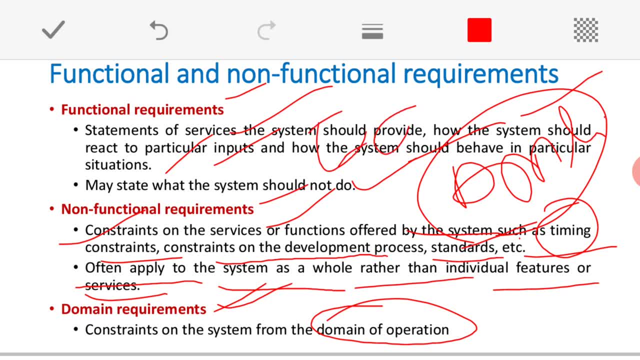 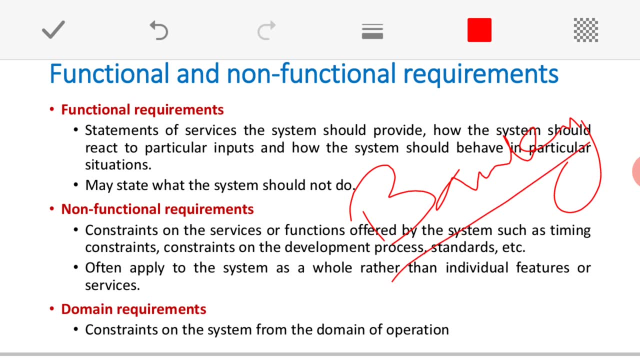 software, it is for the domain of education system, So education is one domain ok. Similarly, today if I am using one banking software, so that will be used for what banking domain? So banking itself is what one domain ok. And today if I am using one software for hospital purpose, that is hospital management. 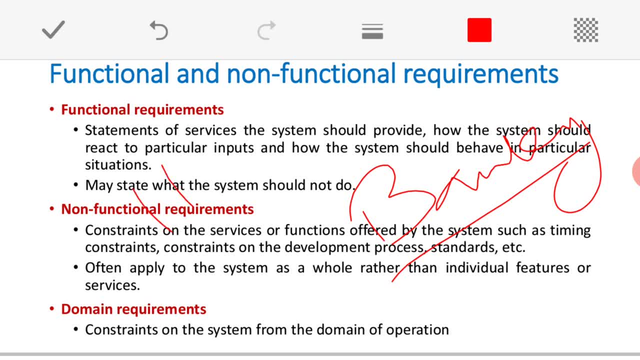 software, then hospital itself is what one domain. ok, Then I might be using another software for railway department. then the railway department itself is what one domain? So it means that you take that education, ok, that hospital, railway department or banking sector, all these 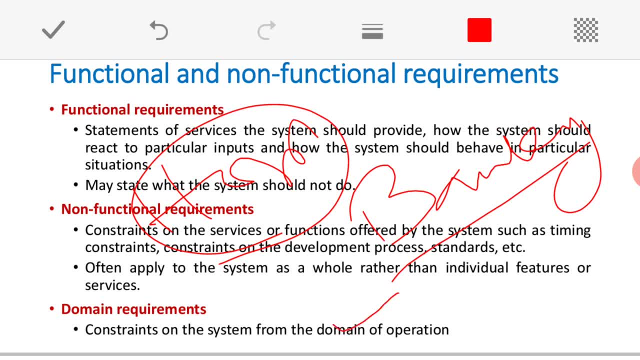 comes under a category of what their own separate domains, And every software is going to provide the functionalities and services with respect to that particular domain is concerned. ok, And here the meaning of the domain requirement means sometimes we need to define the requirements based on that domain area. domain area of. 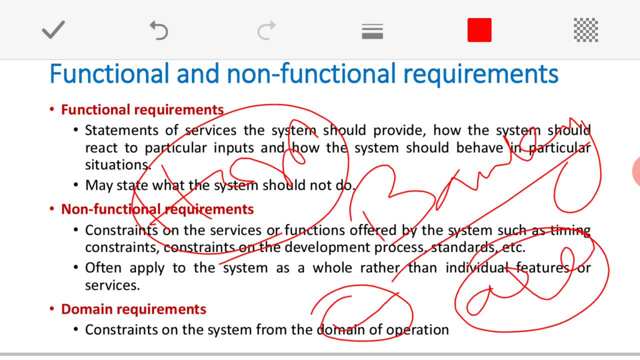 what the where my software is being, what used. See, for example, say, when I am talking about the banking software: ok, So there are so many things that we need to deal. come up with banking domain, the terminologies and functionalities. Is it clear? Credit debit: ok, simple interest. 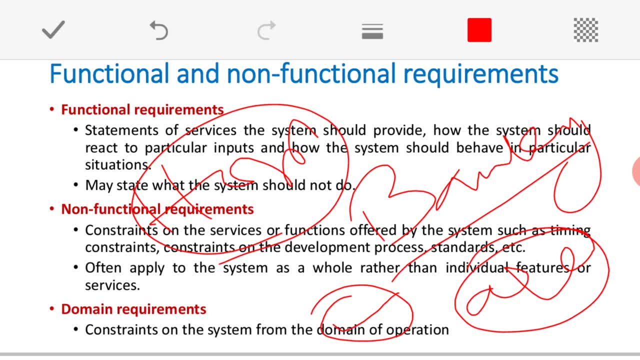 compound interest, ok. sanctioning the loan, cancel of the loan or money transfer within the bank or different banks, see there. So here there are so many things which are purely related to the banking domain means banking sector. So as a common person I may not understand. 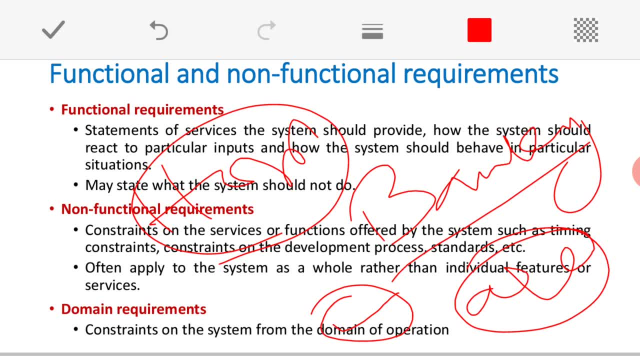 or as a software engineer, I may not be knowing that- how the bank will work, Is it clear? So most of the requirement that should come from the people who are actually working in the bank. So a common end user cannot come and say that, so this should be a requirement. 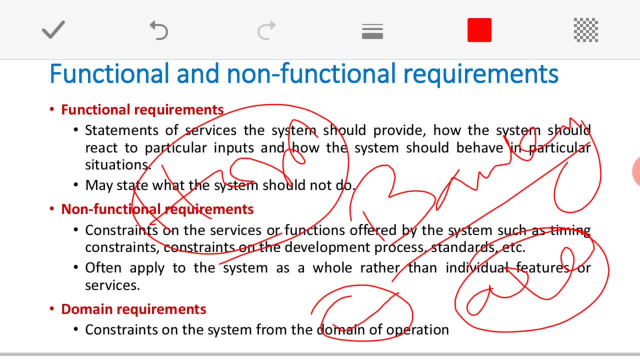 for a banking software, because he is not having an expertise in that particular bank and he may not be knowing that how the bank will work. ok, So today, if I am developing one software for a railway department, I should know that how the railway department will. 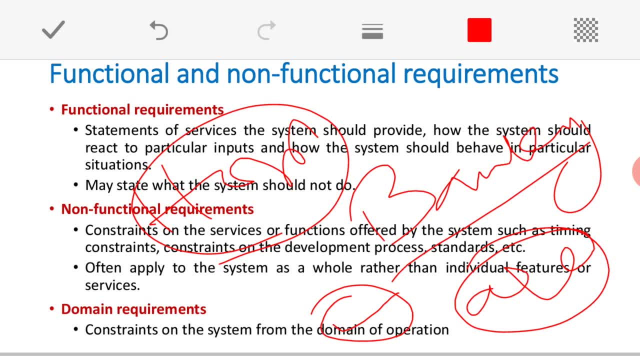 work ok. So I do not know how the station master is working in every station. how many of us know that 金箱? until and unless I know how that particular the area will work in that particular area, So I we cannot define the requirements for such type of software. So that is the reason. 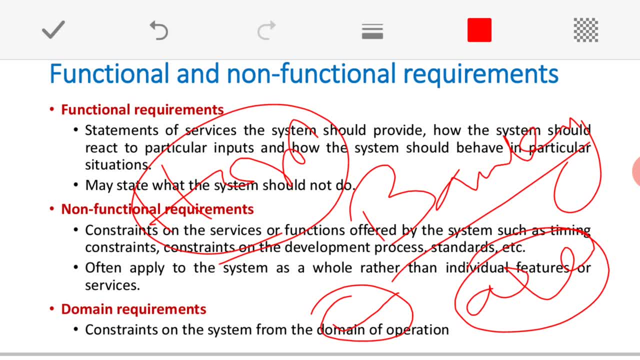 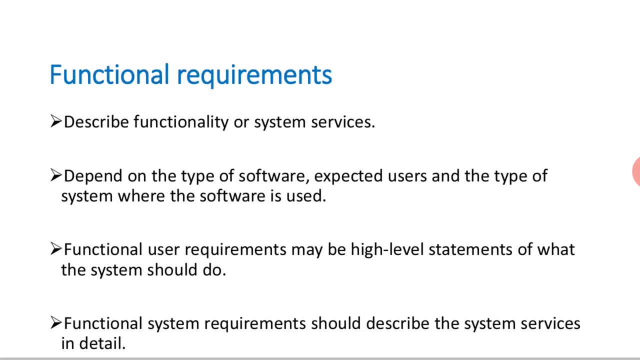 that most of the software requirements will come from that domain area. they are called as what the domain requirements. it is clear, ok, So we will discuss one by one here. So let us start with the functional requirements. So the name itself indicates functional requirement. 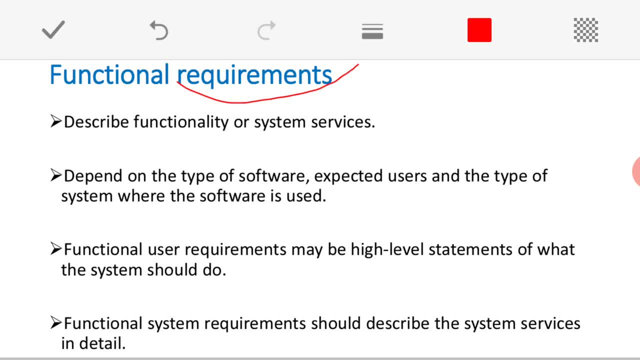 means the requirement which will provide what a sort of functionalities the services. ok, So normally the functional requirements are going to describe what the functionality or what the system services, that software is supposed to provide to the end users or the variety of stakeholders. ok, And these requirements always depends on what the type of the software 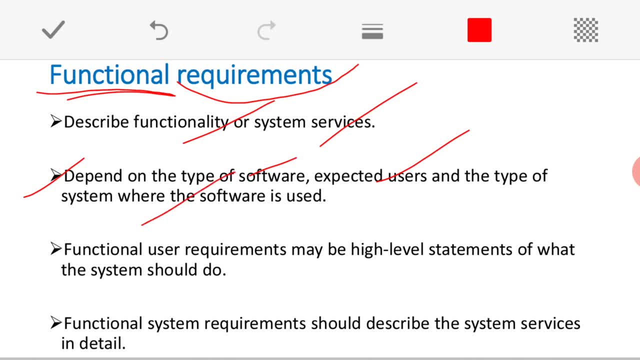 and the expected online customer service requests. So the first thing that is going to have to be understood. So the first thing that we have to be understood is that what is the actual service? Graeme is the customer service, users and also the type of the system where the software is, what used? ok, so it depends. 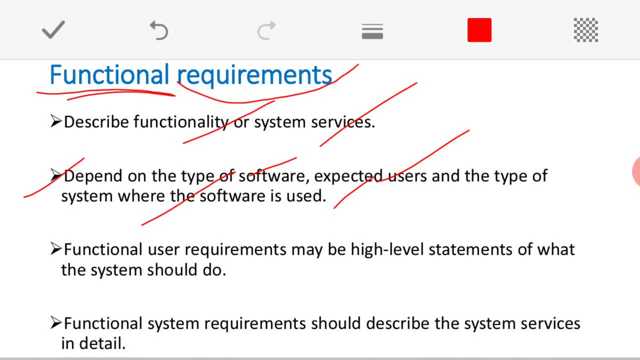 on that environment, the nature under which you are supposed to use that the. it is also depends on what the expectations of that particular user, the type of the users and also the type of the software. clear, and another point is for the functional user requirements may be what the high level statement, because they are functional requirement but which has been 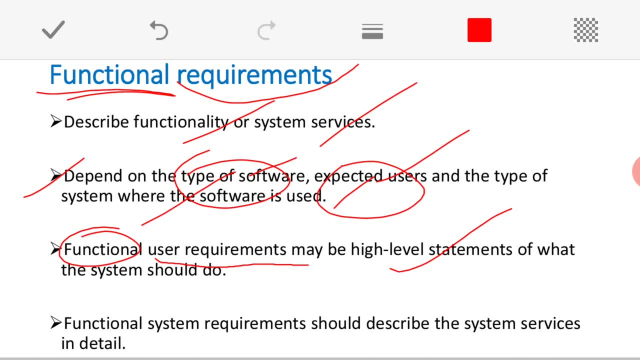 used, defined for what users, so that we have already discussed user requirements- will be always at the high level statements of what the system should do, ok, and at the same time, the same functional requirement as a part of system specification, system requirements. then they will be get described, the system services, in detail. it is very important that 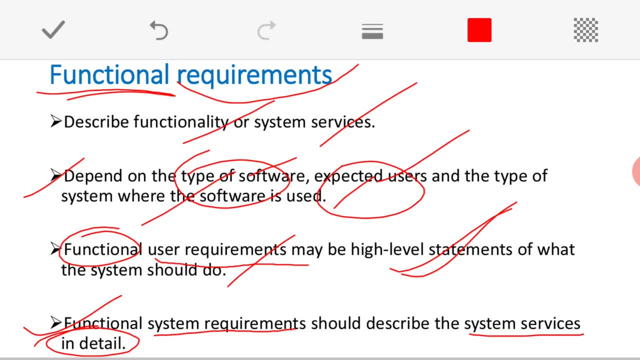 also, we have already discussed the difference between user requirements and what, Ok, The system requires. system requirements are always what in detail, and they are more technical perspective, mathematical perspective, and every detail will be get incorporated while defining the requirements are concerned. ok, so now just have a look at the functional requirements. 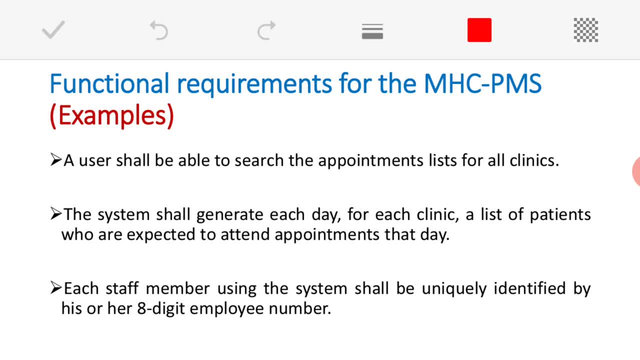 examples here. see, for example, see if I take an example of a MHC PMS, that is, mental health clinic patient management software, the case study that we have already discussed in one of the previous video. ok, Just have a look at my first example of the functional requirement. here a user shall be. 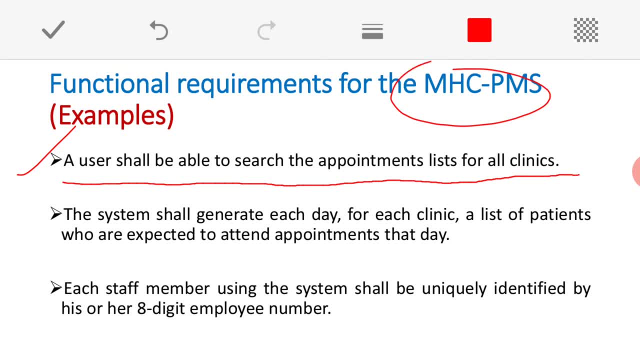 able to search the appointments lists for all clinics. So means so here this MHC PMS software should provide a facility for the end users to search for what an appointments, whether the appointment is available or not. ok, for all the clinics. ok, so you should not put any restriction on the patient to take the appointments here. 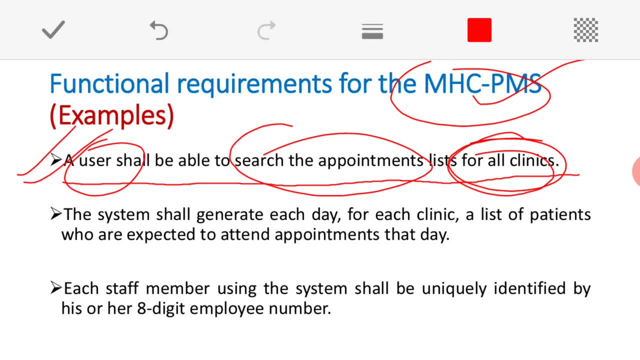 Ok, That is so this is one user requirement. then it is very easy to identify the user. the functional requirements here, just have a look at here. so here the user shall be able to search. so searching is what one kind of functionality that the software should provide. it is a verb. 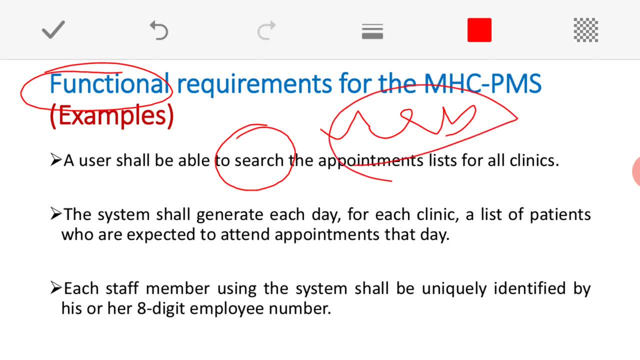 it is very simple to identify that. so wherever we are using the verb while defining the requirement, using our natural language, so that you can treat it as what a functional requirement here, So it should provide a functionality of what? Ok, Ok, Searching functionality. look at the second one the system shall generate. see there it. 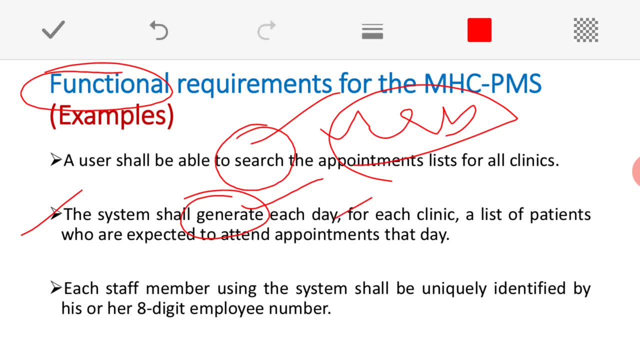 should provide a functionality of what: generating each day, for each clinic, a list of patient who are expected to attend appointments. that means every day. ok, it should provide a list of all the patients who we have taken the appointment of that particular day. So it means that here it is also a what functional requirement. why? because 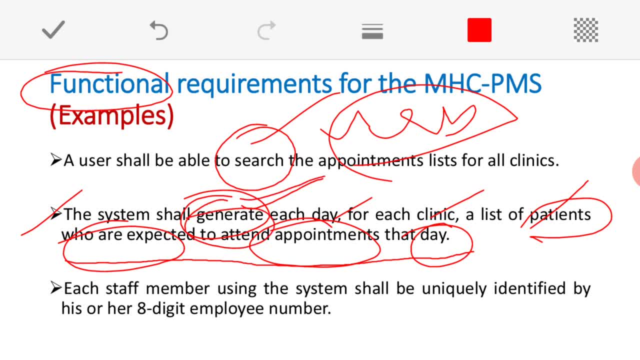 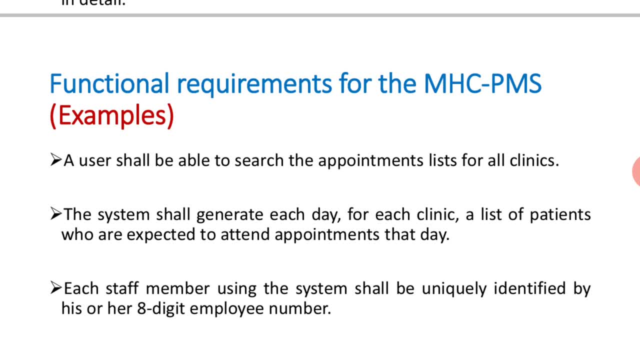 It is going to provide a function, function of what- generating the report, a kind of report, is it clear? look at the another example. each staff using the system shall be uniquely identified. so here it should provide a functionality of what: identification of the authorized staff members using what, using his or her eight digit employee number, assuming that to use. 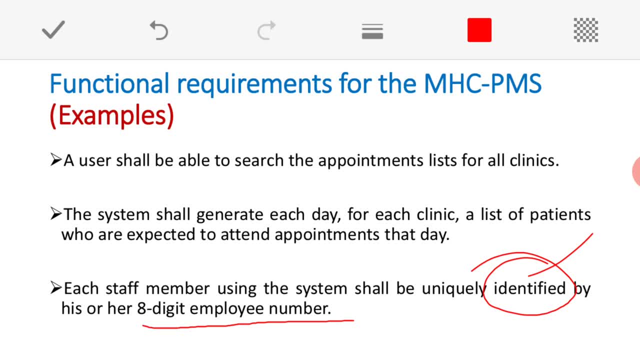 that MHCPMA software, every medical Staff has been given a eight digit employee code. using that number, every employee will be get identified by the software. that is it ok. so here, if you observe, searching, generating, identifying, see there all these a part of what a providing a, a kind of functionality. 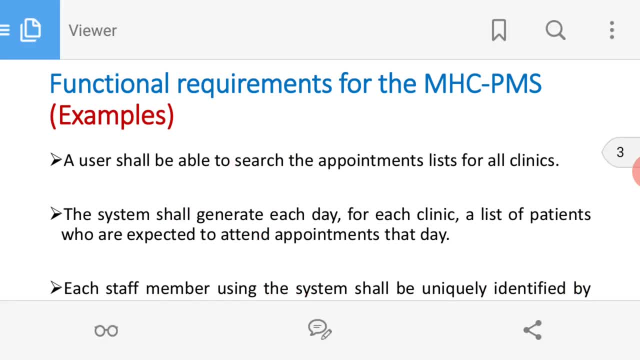 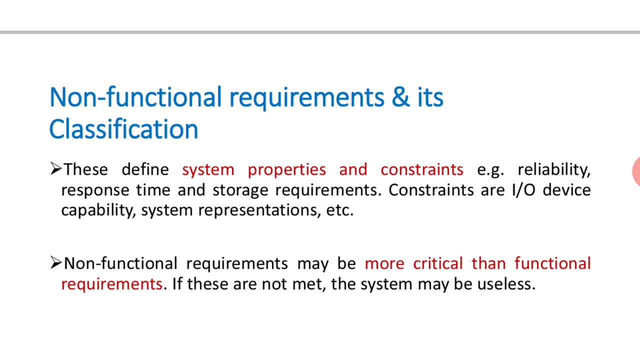 for the end users clear, ok, So now come to the non functional requirements here. ok, and it is a classifications. so basically, as we told just now, the non functional requirement means these are going to define the system properties and constraints, for example, say, reliability of the system, response time of. 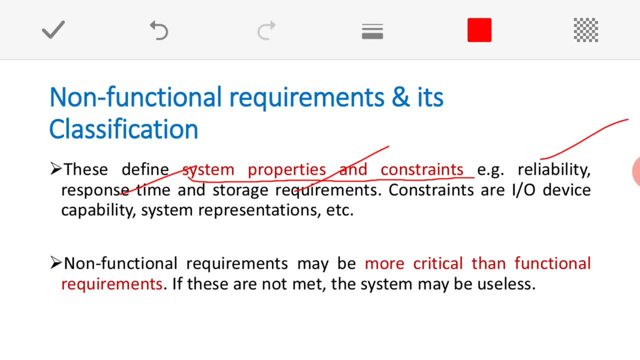 the system storage capacity or the storage requirements or the constraints are like I, O, device capability or system representations, so like this. so with the very important thing is ok, It is very easy to understand The or to differentiate between this functional and non functional. ok, so the name itself indicate: 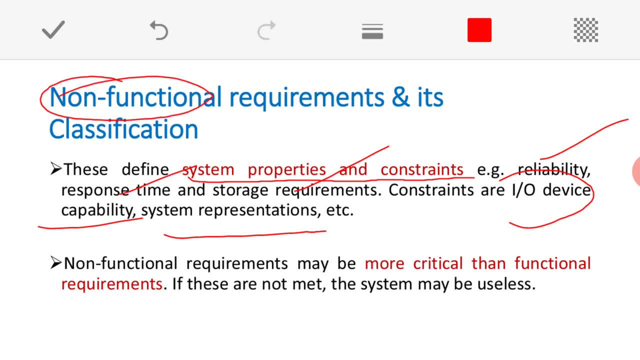 non functional. so here we are not interested saying that the system should provide a kind of functionality here. so here we are talking about the system properties. system properties in the sense what the behavior of the system, ok, see, for example, say when I will say that when I will buy a new mobile I will be talking about my RAM size, size of the RAM, for example. 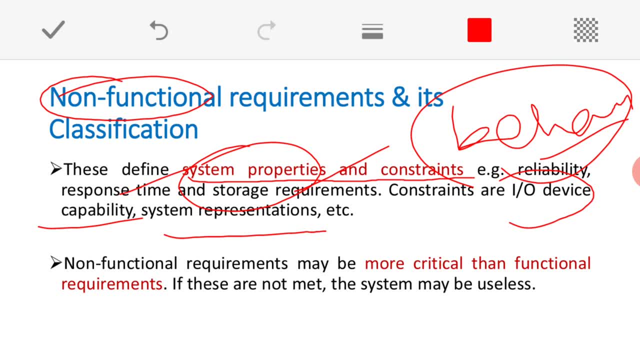 say, My RAM size is 4 GB, so my system is very fast. see there. So here I am talking about what the property of my mobile here, ok, the behavior of my mobile, so that is going to be get defined here, So that that comes under what a non functional requirements. it is clear. see, for example, say: 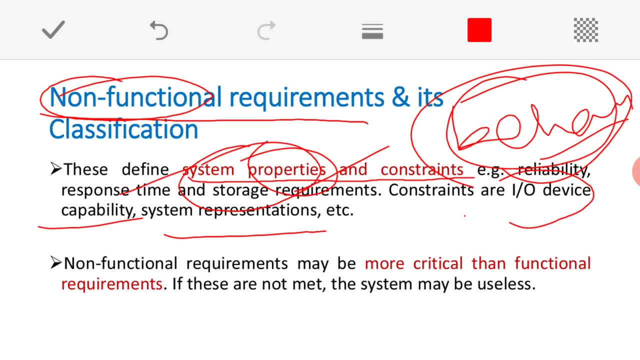 just now we told that one functional requirement, just try to recall- in the previous slide. so what was that? That MHC PMA software should provide a non functional requirements. Ok, The software should provide a search option- ok. now the question comes here for the search. 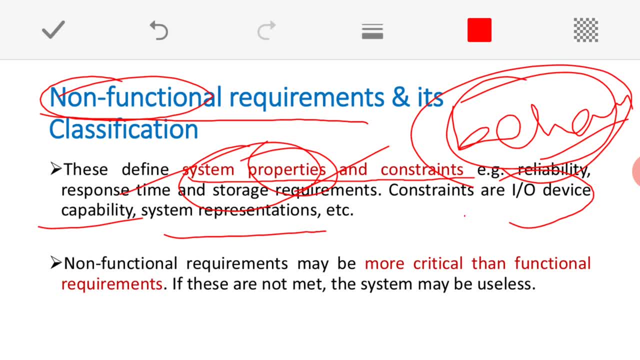 option. ok, if I want to search for any clinic, how much time it will take to display the list of the clinics, whether it will take 5 minutes, 10 minutes or 1 hour. so that is going to talk about the response time of the software. ok, today, if you search with any keyword in: 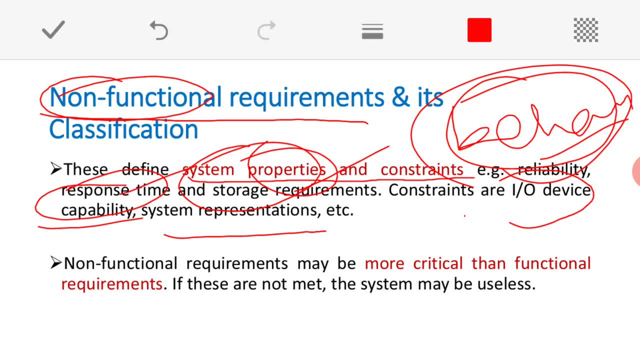 the google so it will make a list of latch together websites with that particular keyword within a fraction of second. See there, See the response time of that particular search engine. ok, so that will talk about the performance of that particular search engine. it will never say that you come after 1 hour, it is clear. 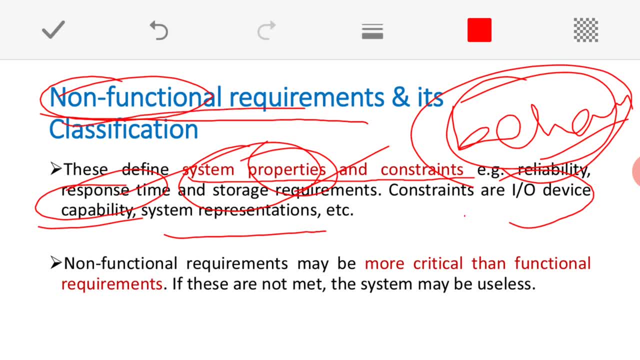 so that that is going to define what the non functional requirements. ok, hope this is cleared here. and always the non functional requirement may be what they are, the more they are more critical than what the functional requirement always remember for any software is concerned. ok, Irrespective of 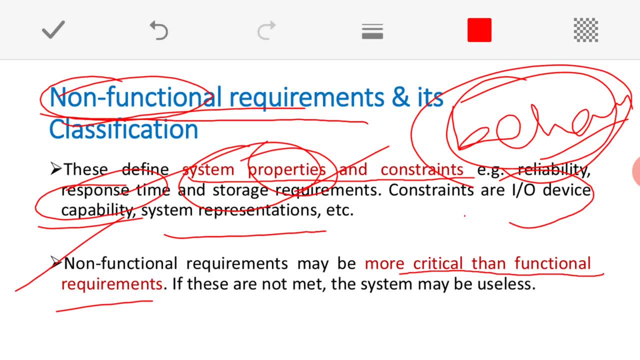 Ok, Variety of functionalities that my software is going to provide to the end user. ok, the non functional requirements here are very, very important than what the functional requirements. why? because, ok, even though if your software is going to provide a variety of very good functional requirements, if your software is not reliable, if your software is not efficient, 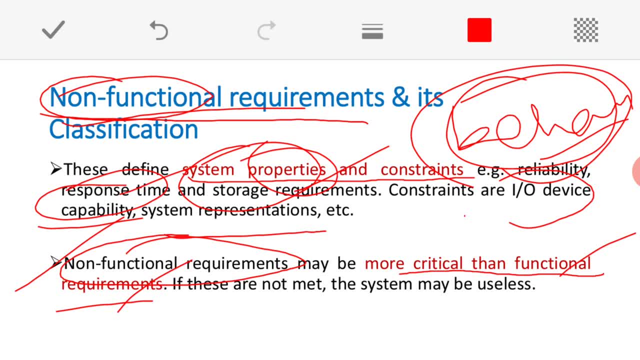 if your software performance is not good, then automatically that software is going to be get plop. No, No, No, It is for that you are talking about. your software is going to work ok If, for example, so today- you are using, there are many apps related to what the money transfers. 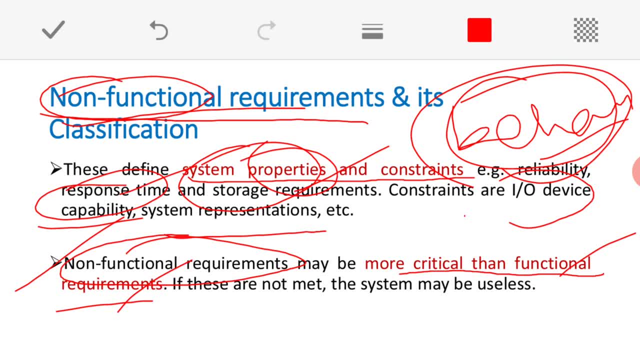 you are going to pay your money, So maybe I am going to make a payment. There are so many apps are available- ok, So today, the functionalities The apps are going to provide are excellent, but the very important thing is the non functional requirement is ok. security and safety with respect to your money. 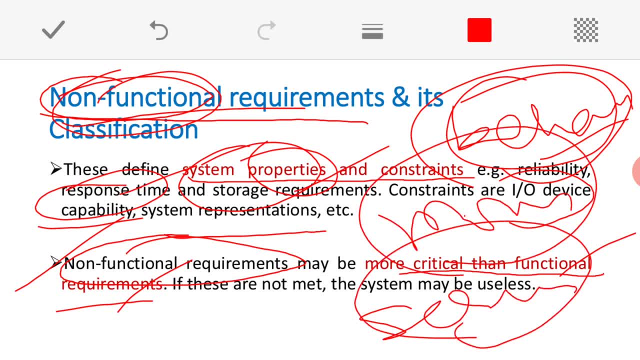 With what guarantee all of you are going to trust this? Are you going to trust this? Ok, To our right hand, that apps, ok. whether your money is safe in all those apps, ok, now, what is the guarantee that the third person will come and what hack that? so that is called as what security and? 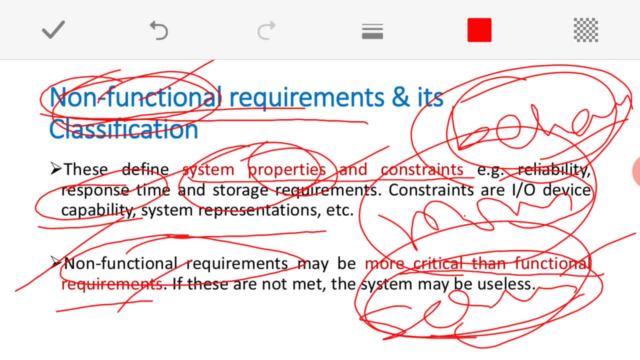 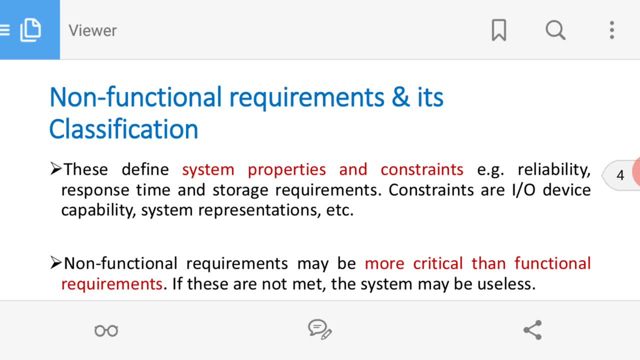 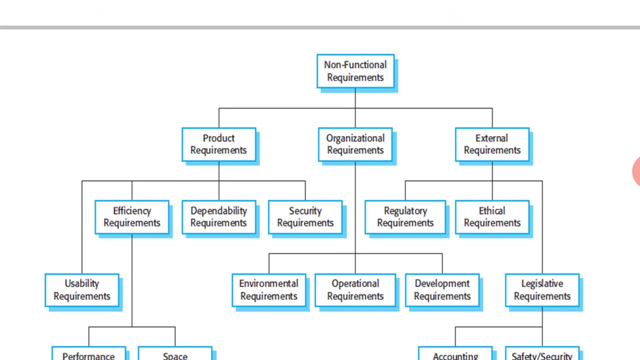 safety. so security and safety comes under what? the non functional requirement? they are not the functionalities here. ok, so hope all of you have understood the very basic definition and the concept of this non functional requirements. so now the another important topic here, that is, the classification of non functional requirements. so once again, ah see there our requirements. 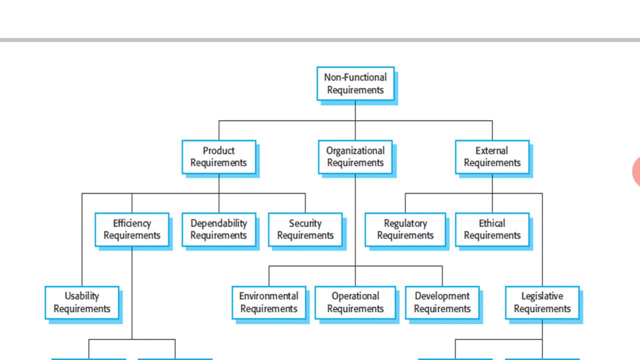 are themselves will be classified into two types: functional and non functional. now, within the non functional requirements, once again, there are three types of requirements. ok, so my non functional requirement may be called as a product requirement, or it may be an organizational requirement, or it may be an external requirements. ok, so now just have a look at the definition. 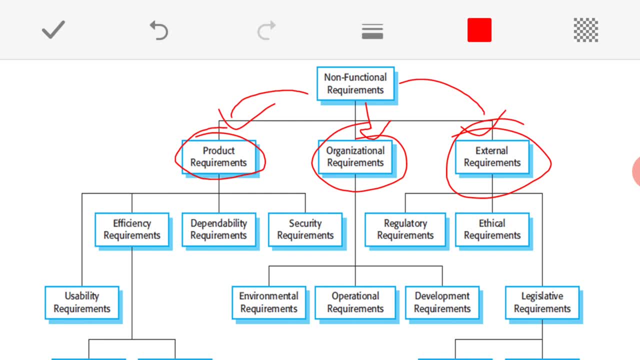 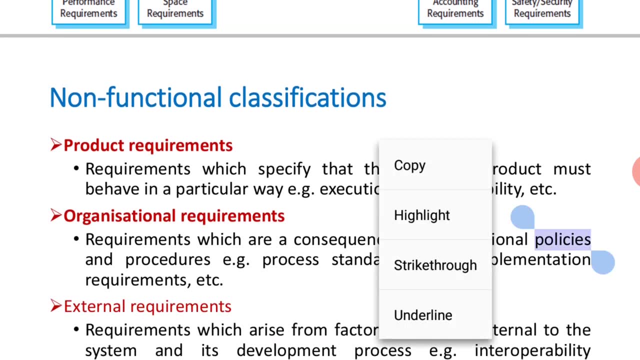 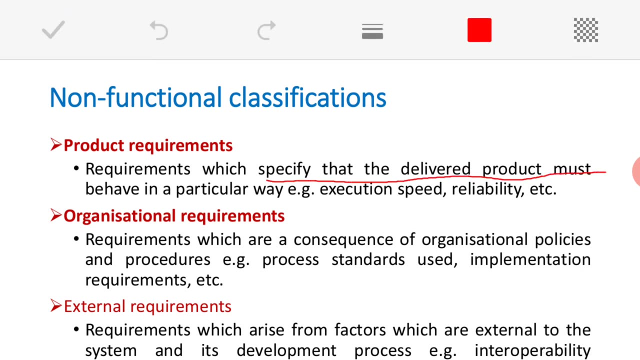 of all these three types. what is product requirement, what is organizational requirement and what is external requirement? just have a look at here. so what are the product requirements here? so the product requirement is nothing but what. these are the requirement which specify that the delivered product must. 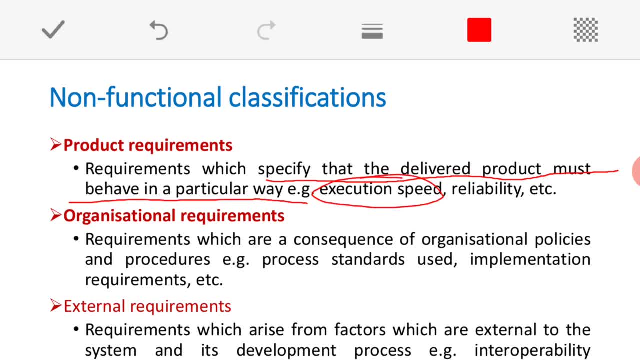 behave in a particular way. example: its execution speed, its reliability, its availability, its security. safety means if you are purely talking about the behavior of your product or behavior of your software, then such requirements are called as what The product requirements see. for example say: imagine that I am. I am developing one software. 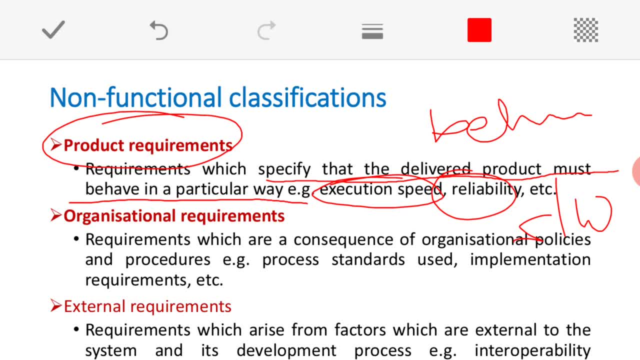 and I will tell that my requirement will be ok. the software, once it is get installed, it should not consume more than 50 MB memory, see here. so here I am talking about the size, the volume of the memory that it is going to consume. so So that that that is what the product requirement it is going to talk about the size of the 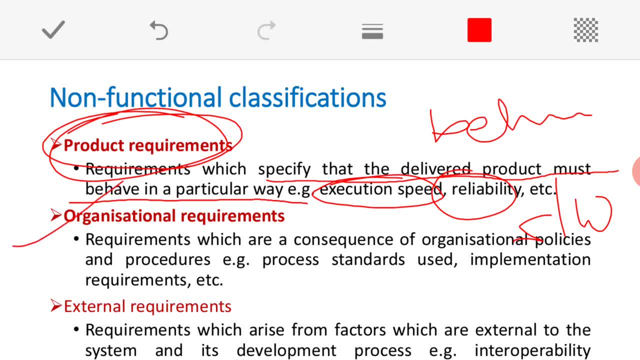 software here, is it clear? ok, Then second one is: what organizational requirement- see the name itself- indicates here the requirement is non functional, but it is related to what an organization. organization means, the company or the organization under which the software is being, what developed. 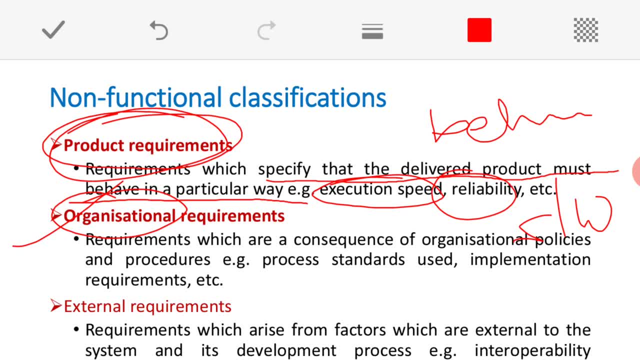 So sometimes some requirements are coming from that organization itself. So examples, for example: see here: these are the requirements which are consequences of organization policy, organization procedures. See, for example, say, if a software is get developed in XYZ company and if that XYZ company. 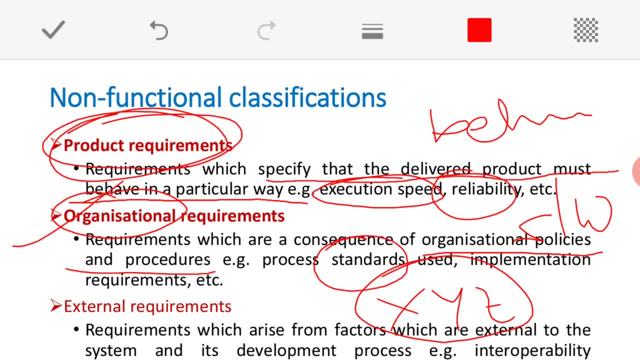 is supposed to follow some sort of process standards, and we have to follow this standard. Whenever I am designing, whenever I am writing a code for the software, that software has to follow that organizational policy because of which it has to undergo a process. So some process standards, some standard has to be followed. ok, some implementation. 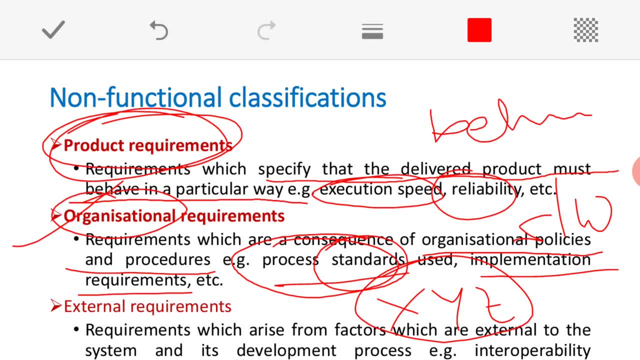 requirements. ok, So it means that every organization is having its own rules and regulations, its own policies, So that we need to follow as a requirement they comes on. that is called organizational requirements. Then the third one is what external requirement the name purely indicate they are. these are: 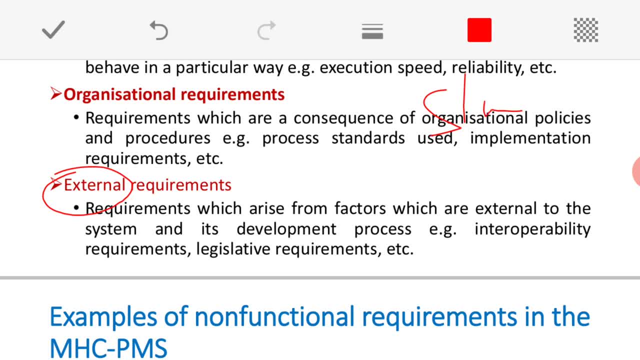 external means. they are not related to the software product, they are not related to the software which is being developed in that organization. So that is what organizational requirements are. So that is what organizational requirements are. So that is what organizational requirements are, which is third part, that is, the external. 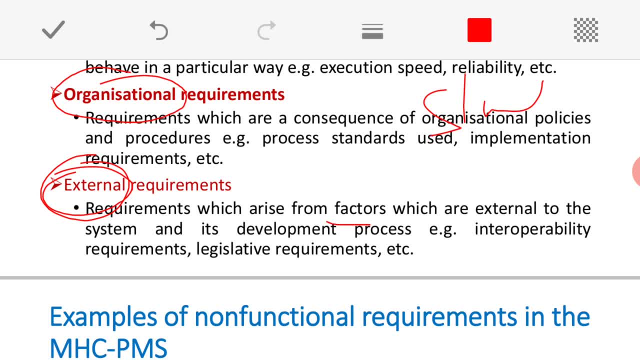 mean some requirement which are going to come from what, the factors which are external to the system, and it is what? development process Example: interoperability requirements or legislative requirements. see, for example, say, today you take any system or any software that is being developed by any company. they have to fulfill. 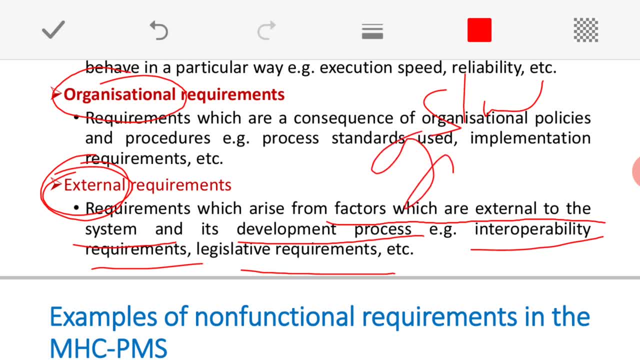 some government policy and government rules. So where government is what? An external body? So it is not a. so government is not a software company. Government itself is not a software. but as a software company, if it is developing one software, it has to follow the government rules and regulations. 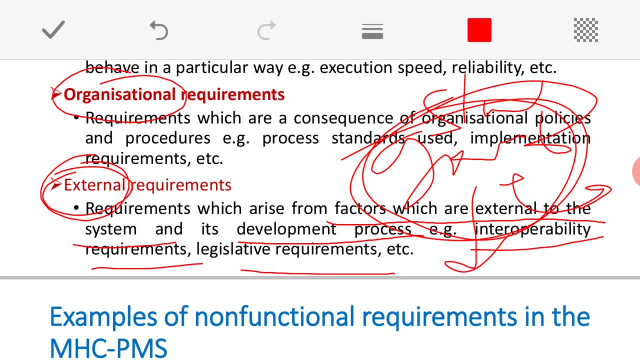 For example, say, today we are all using that example. I told money transfer apps that we are using. is it clear? So every app should work with some government policies and rules and regulations why? Because every banking activity that we are going to do online, it should be get regulated. 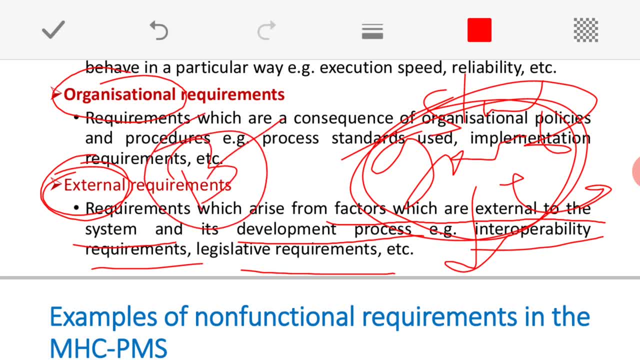 by the nationalized bank. banks will be there and every bank is controlled by what RBI. So where RBI is, what An external body? So some rules and regulations and some requirements are coming from what That RBI See, for example, today, if you take an example of our engineering college, is it clear? 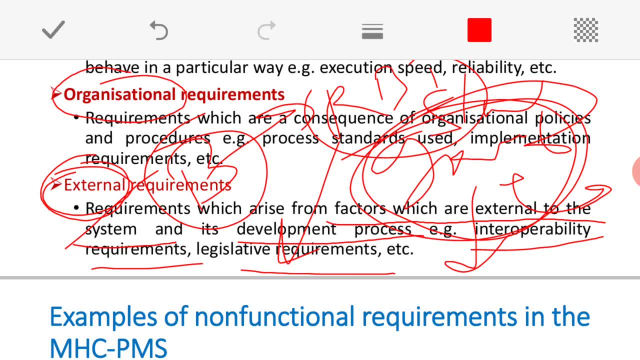 So as an engineering college it will be get managed by our organization. our management will be there, But that our college and management Both will be get controlled by what A university That university is, what An external entity here, And this university is having its own rules and regulations. 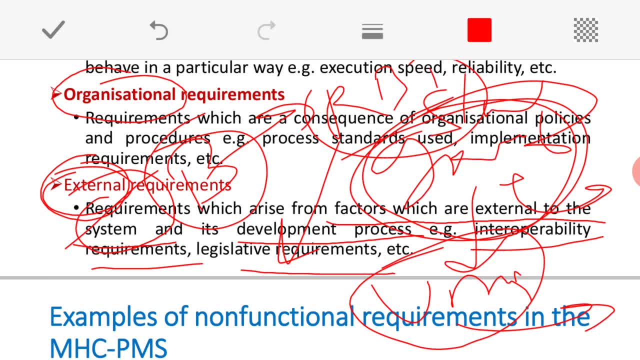 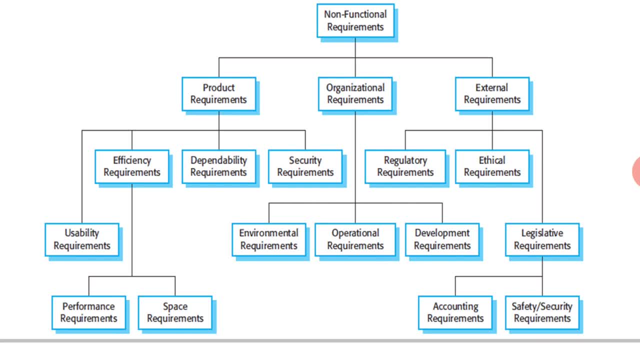 Because of that rules and regulations, some requirements will be get emerged. is it clear? So that is what an external requirement- and this is a big table- is present. over here you can come across with a different examples. For example, say, product requirement means efficiency, dependability- that you know, dependability. 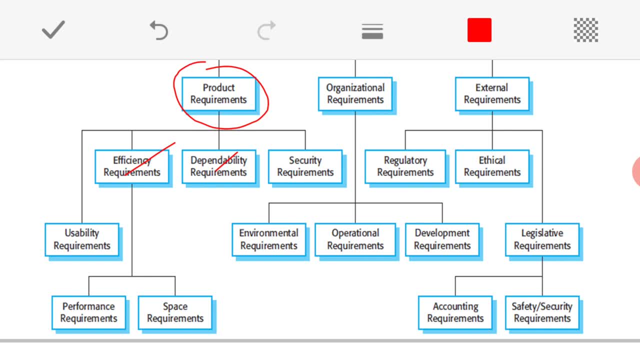 means what? Reliability, reliability, safety, security and within the efficiency. once again, you can classify the requirements. Either it may be performance related or it may be what Space requirements And regarding with the organization is concerned. just have a look at that. either it may be. 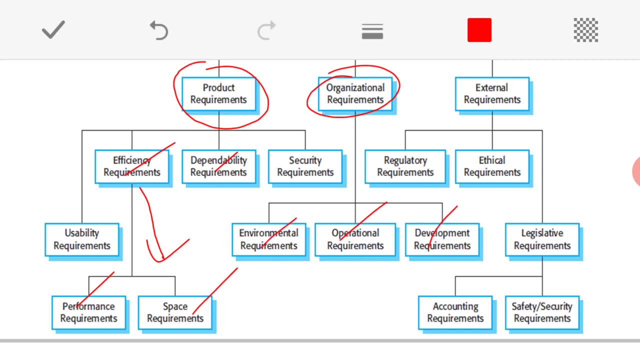 operational requirement or development requirements or what Environmental requirement, See these type of requirements are defined by whom, The organization under which the software is to be get developed and with respect to external are concerned. Now I told, for example, say it may be legislative means. for example, say it may be an accounting. 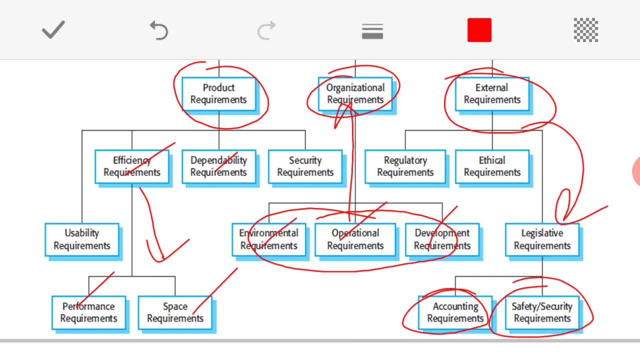 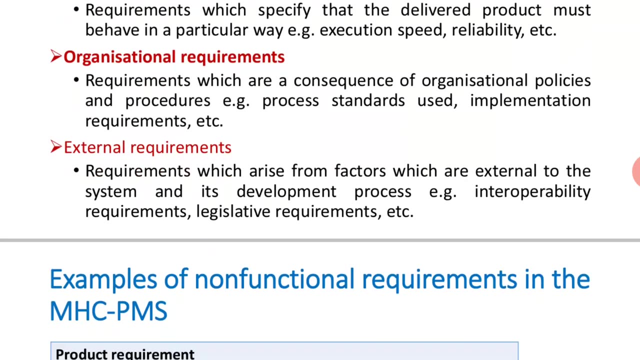 related, or it may be safety, and what Security related. is it clear? So all these requirements are going to be get defined by what? An external entity or a third party? is it clear? So just do remember all these examples And just have a look at one example over here. that is the non-functional requirement example. 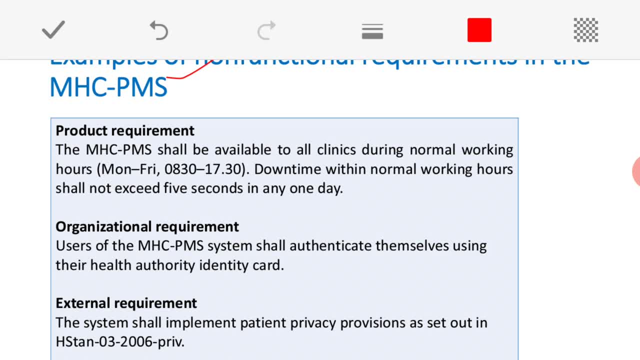 for MSC PMS. once again, The case study that we have already discussed, For example, say product requirement. see there how the product requirement can be get defined here. The MSC PMS shall be available to all clients during normal working hours. Normal working hour means the working day from Monday to Friday, from morning 8.30 to 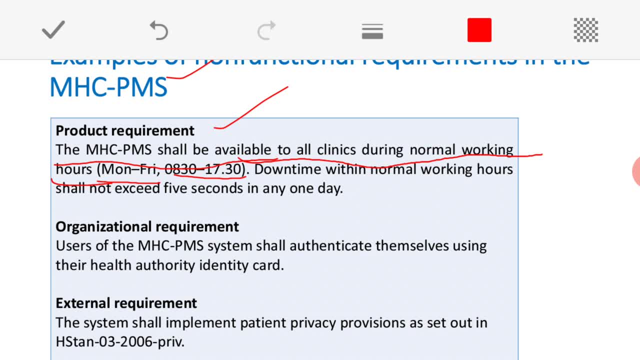 5.30, and also it has been mentioned that the downtime within these normal working hours shall not exceed 5 seconds in any one day. So this is one example. So this is my product requirement. See, this is a non-functional requirement, first of all, but this comes under what? 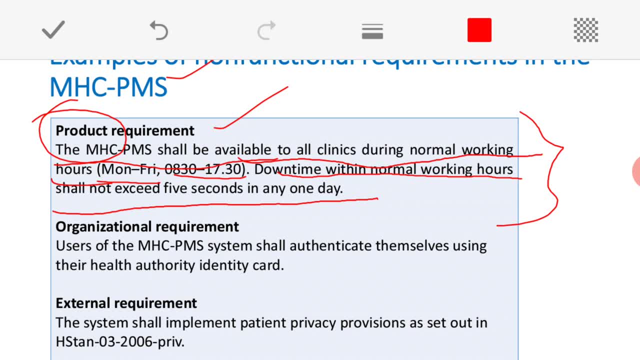 It is going to describe the behavior of the product, the system property, the property of that MSC, PMS. it is going to define. is it clear here, And clearly it is mentioned that, see there, this is going to talk about the availability of the system here. 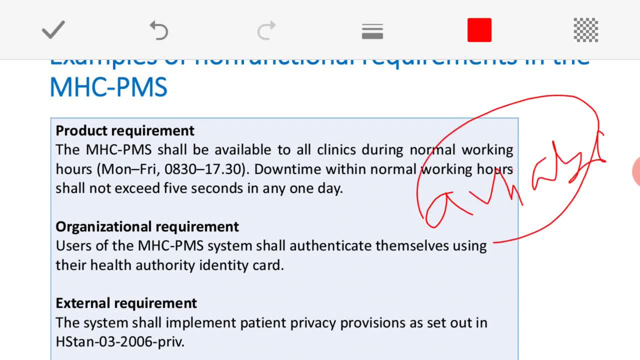 This is going to talk about what Availability means. the system should be available always for all, the Monday to Friday. So this is going to talk about the availability of the system here. This is going to talk about what Availability, Availability, Availability from Friday from morning 8.30 to 5.30, and even during its normal hours. 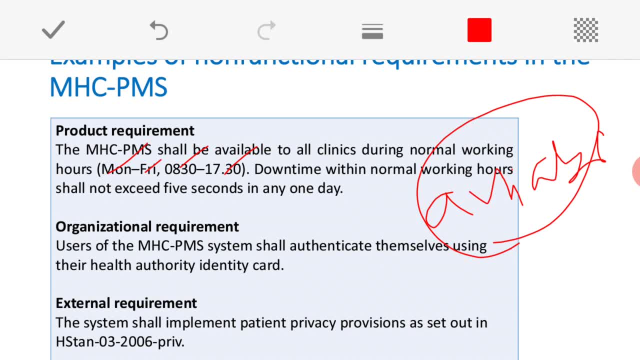 if the system is going to be get down due to some server problem or some internet problem or something else, then there should not exceed 5 seconds. See that even he is going to say that. even 5 seconds also the system should means the. 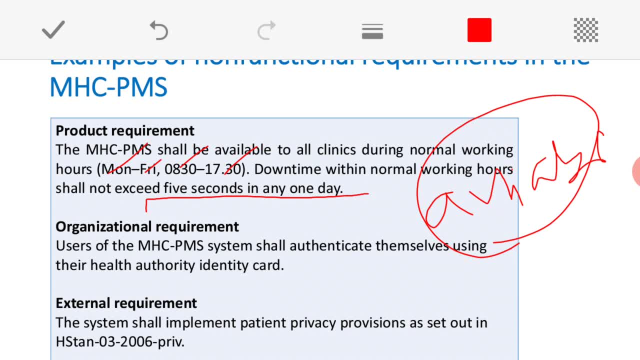 software should not say that today the software service is not available. Then the second example is organisational. organisational requirement means the users of MSC, PMS, PMA system shall authenticate themselves using the health authority identity card. See there, See, this is also a non-functional requirement. but that comes under what organization? why? 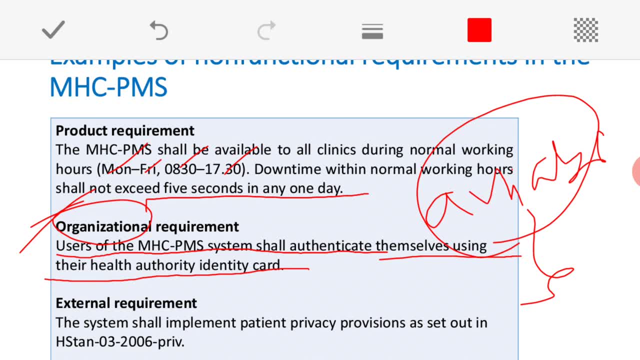 because every authorized user should be get authenticated by what an authority of identity card- health identity card- who is going to give that? this is given by the organization, So that is why that comes under what an organizational. then the third one, external requirement. So here the system shall implement the patient privacy provision as set out in some standard. 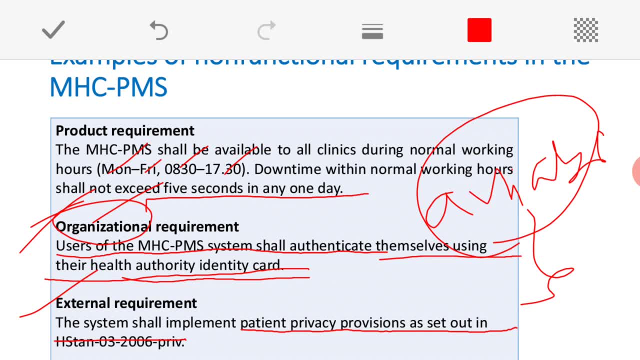 number that we have mentioned just for example. So here this patient privacy is defined by some rules and regulations as per the government norms, because government has clearly told that whenever you are dealing with the hospital is concerned, every record of the patient should be kept confidential. that is called what patient? 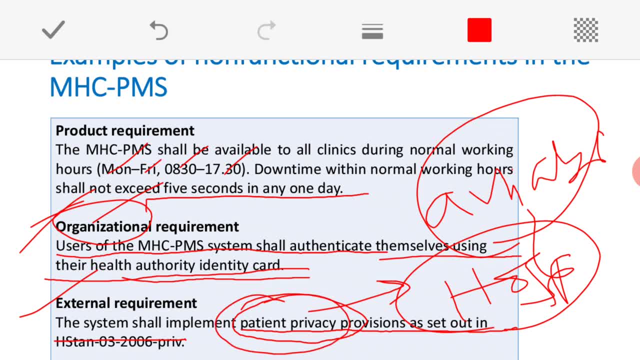 privacy. You cannot disclose the history of the patient to some unauthorized person. so that is against to the law of the government. So it will never happen by any hospital. always do remember: if you go and ask the history of the patient first, they will ask you your authority. 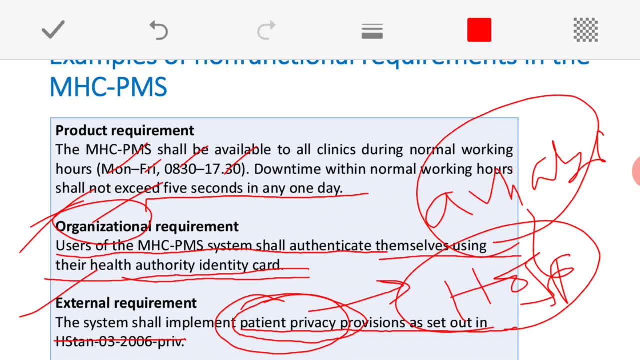 Except that patient or the exact relative of the patient, the patient details will not be given to any unauthorized person. that is called the maintaining the privacy of the patient. So this is the third one. external requirement is coming from where the external? because it is that policy, defined by the government itself, health department is going to define. 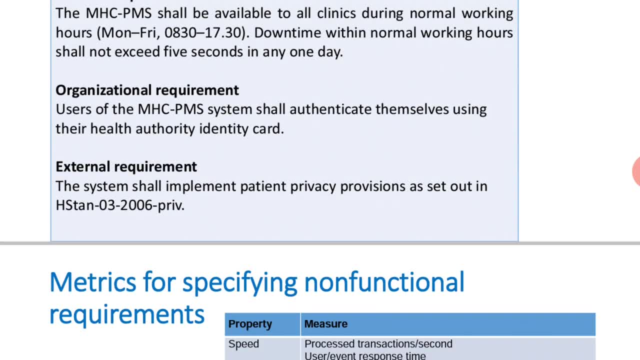 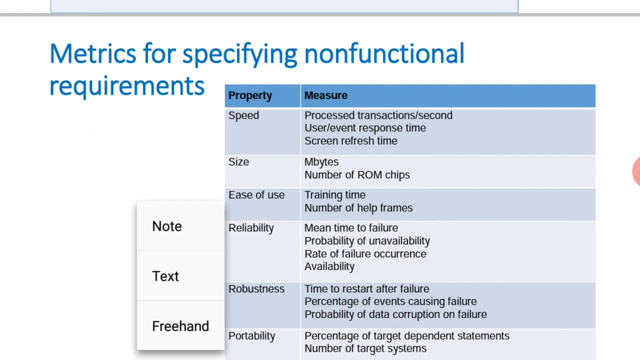 this part, is it clear? So these are the examples here. ok, Now finally just have a look at here some of the metrics for specifying the non-functional requirement. So here it is very difficult to measure this. non-functional requirements means see it and also prove the prove. proving is also not so easy. 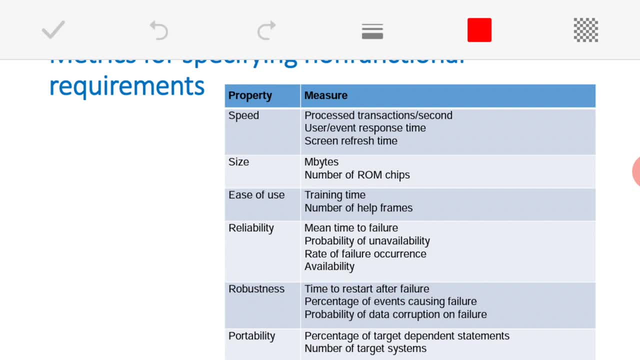 So today, if you develop one software and you are going to tell that my software is 100% high performance, How we will prove that and how we will measure that your performance is 100% and how we will measure that your availability is 100%. ok, why? because there are no specific measuring. 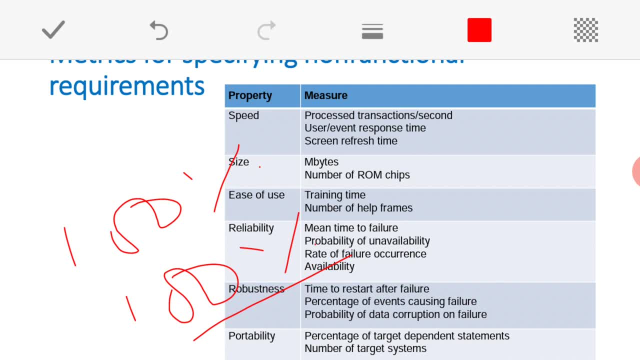 quantities are available, that metrics are available. ok, so that is why here we are going to come up with our own Set of metrics which will help us to measure what our non-functional requirements here just have a look at here. So these are the properties and these are the measuring metrics. see, for example, say: 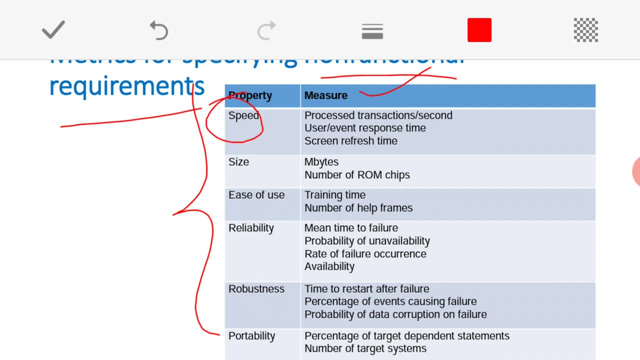 when I am talking about the speed of the software. the speed will be always measured in terms of what the transactions per second, or user events or response time and the screen refresh time. these are the some measuring metrics with which I can measure what the speed similarly size. 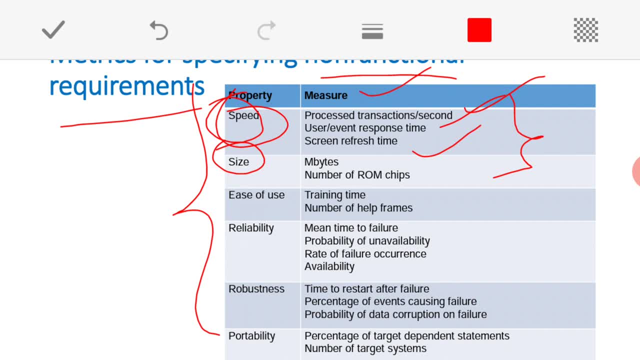 So how we can measure the size memory. for example, say how we will define the size of the memory there, that is, in terms of megabytes, gigabytes, terabytes, or in terms of the number of memory chips that you might be used. then, for example, say how we are going to measure. 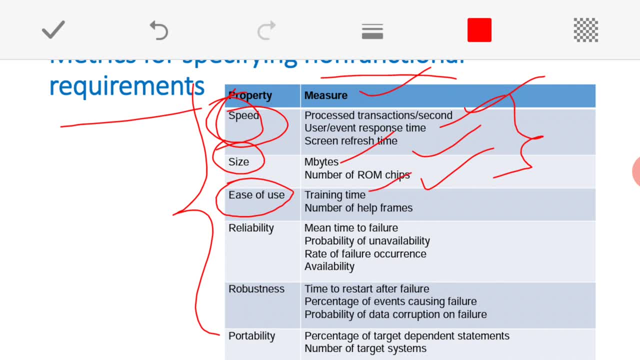 the ease of use. ease of use will be always measured with an example of the training time required. see, for example: say, there is a software A is there and a software B is there, if the A will take 10 days to learn and B will take 5 days to learn. 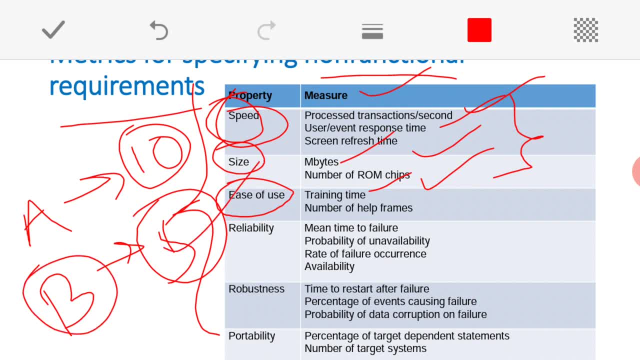 Then which one? easy to learn here, the software B. that is ease of use. why? because the software can be learned within 5 days. ok, So training time which is required. based on that I can define the ease of use. similarly, the number of help frames means whenever you are using the software there, normally you 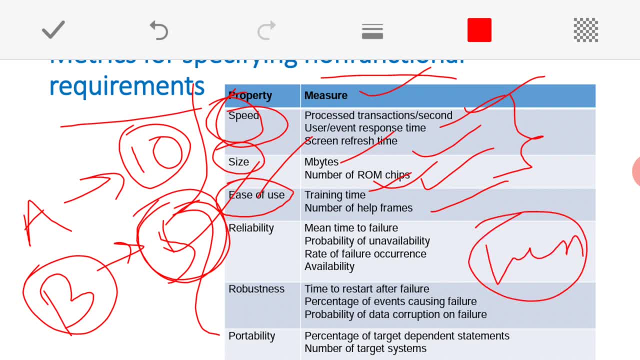 might have seen, there will be an help desk, will be there. so it will be useful for the end user that how to use that software. so, based on the quality of that help, that help frames, So say that the you can measure what the ease of use. then, similarly, how you are going to 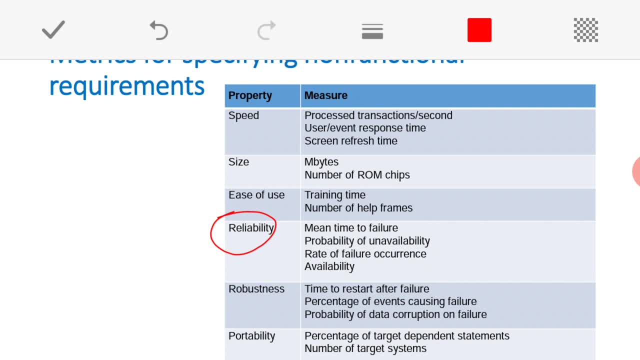 measure the reliability of the software. ok, So that is mean time to failure or probability of unavailability, rate of failure occurrence or what the availability? based on that, you can tell that. what is the percentage of what reliable, whether my software is reliable or not is it clear? for example, say there is a 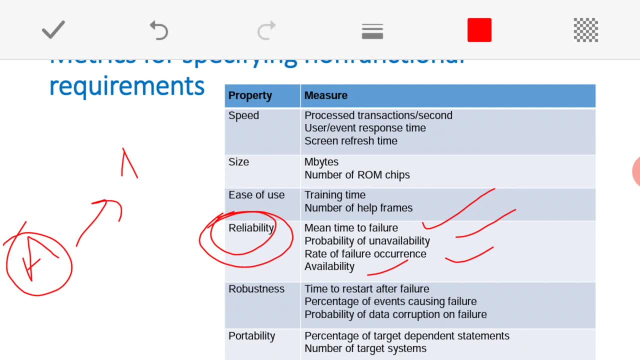 software A. if it is going to be get failed once per day, Ok, Every day, one time at least it will be get failed. then how you can you say that the system is reliable there? no, then automatically ok. Similarly, the robustness: robustness means time to restart after failure means see it.